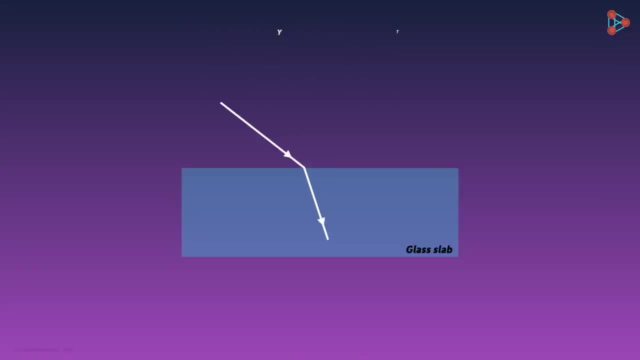 Now this light will bend at the boundary of the two media. Here the two media are air and glass. This bending of light at the boundary of the two media is what we call refraction of light. We see that the light travels from one medium to another. 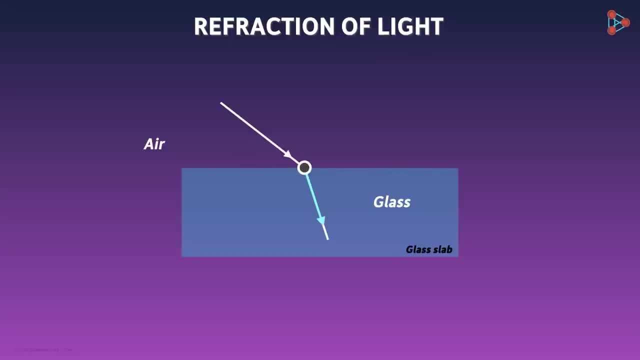 This is called refraction of light. We see that at this point the light bends. It's not going straight. What are these two mediums called? The medium from where the light is incident is called the incident medium, and the medium where refraction occurs is called a refractive medium. 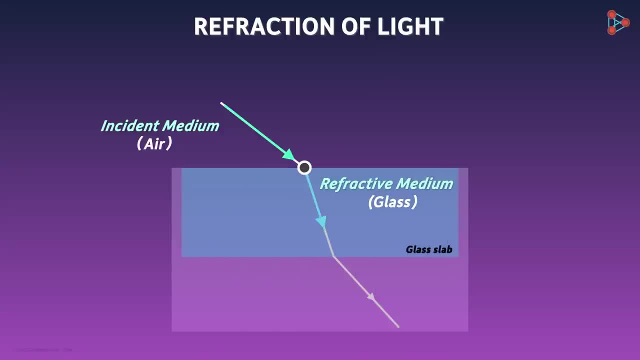 Similarly, here as well, the light is travelling from one medium to another medium. It's from glass to air, And here also, it is incident at an angle, Since we know that air is a transparent medium. Light bends at this boundary and travels through air. 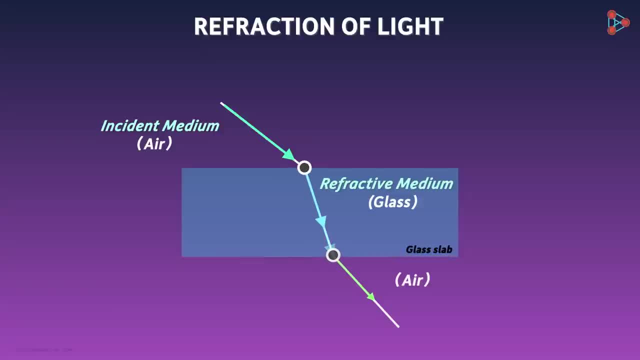 So light refracted at these two points. Let us draw a line perpendicular to the surface at this point of incidence. This line is also called a normal. What is this angle called? It's called the angle of incidence and is denoted by the letter I. 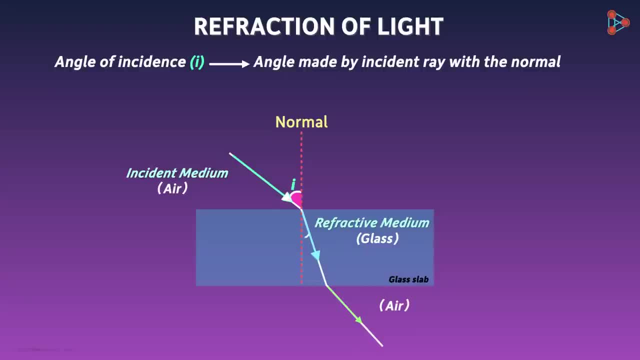 It is an angle made by the incident ray with the normal, And this is the angle made by the refracted ray with the normal, And this is the angle of refraction r. Now there might be various questions that you have. Why does refraction occur? 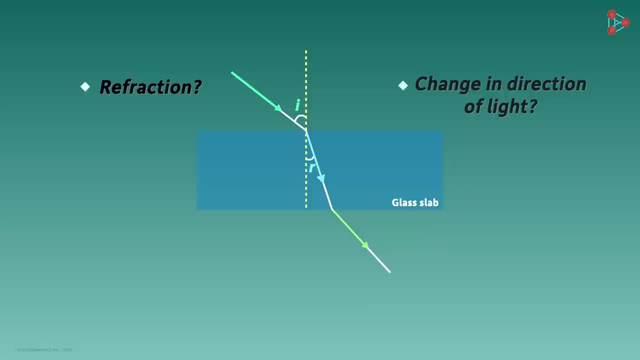 Why does light change its direction after entering another medium at an angle? Why does incident light have to be slant in order to change its direction? Can the refraction occur if the light enters perpendicular to the surface? We will answer all these questions in the coming videos. Thank you for watching.